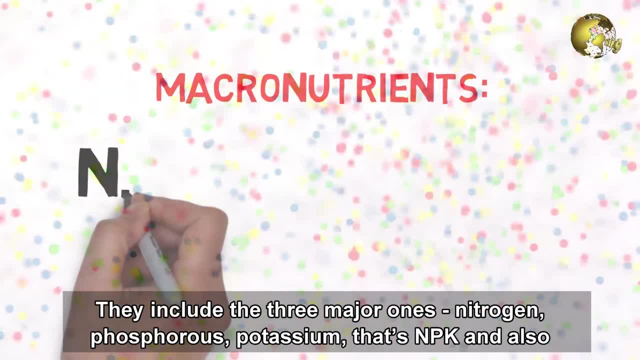 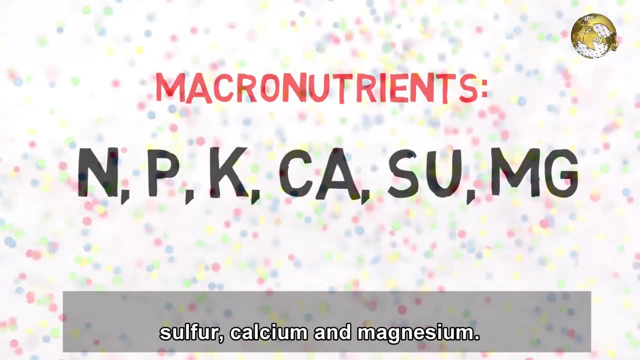 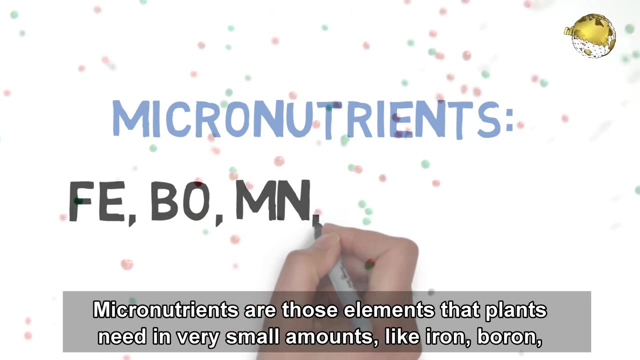 Macronutrients are those elements that are needed in relatively larger amounts. They include the three major ones, ie Nitrogen, Phosphorus and Potassium, and also Sulfur, Calcium and Magnesium. Micronutrients are those elements that plants need in very small amounts, like Iron Boron. 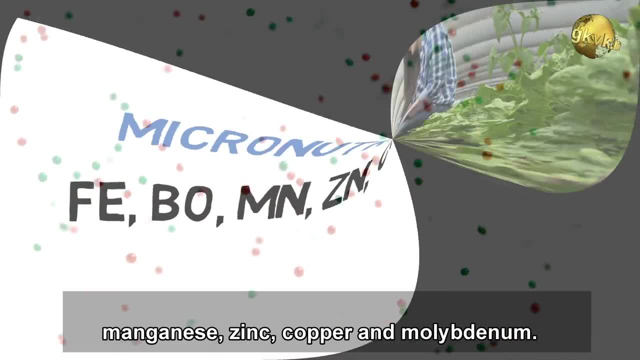 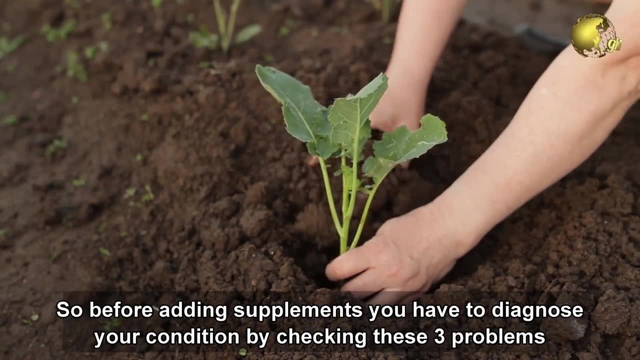 Manganese, Zinc, Copper, Molybdenum, etc. Most of the times, except in container gardening, these nutrients may be present in the soil. So before adding supplements you have to diagnose your condition by checking these three problems or factors. 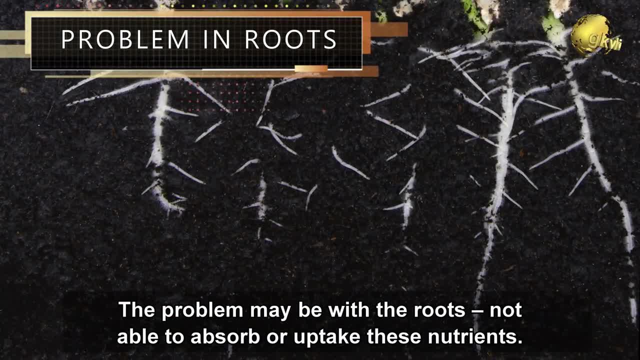 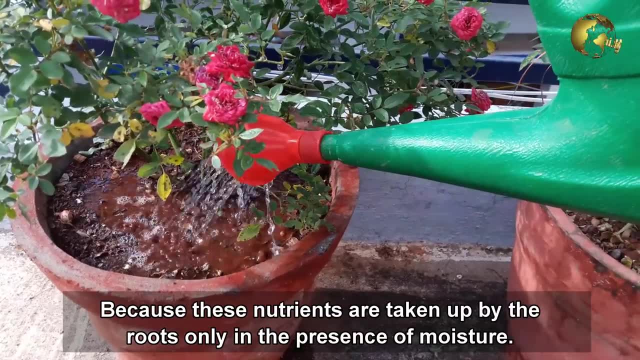 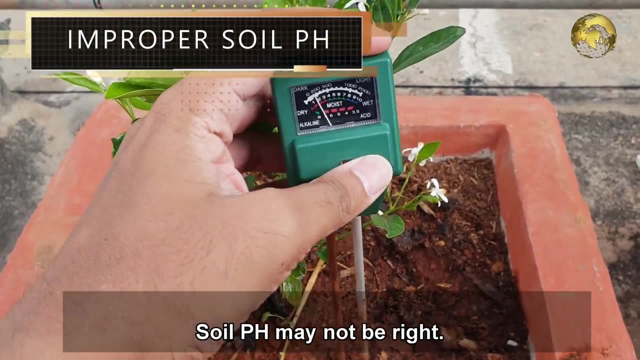 1. The problem may be with the roots not able to absorb or uptake these nutrients. This can be due to root disease or improper watering, Because these nutrients are taken up by the roots only in the presence of moisture. 2. Soil pH may not be right. 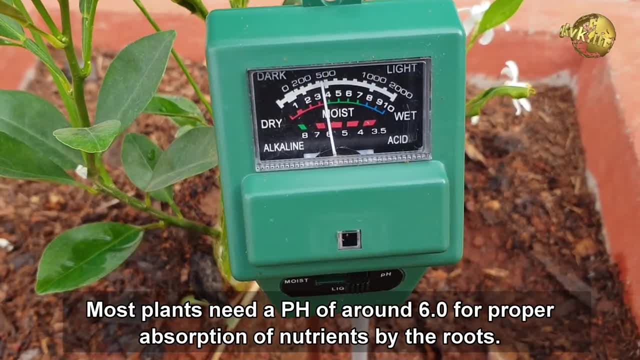 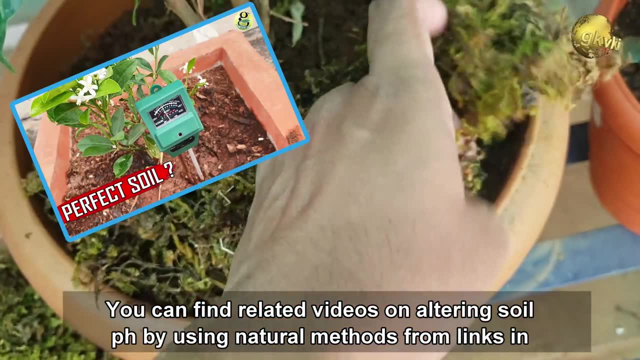 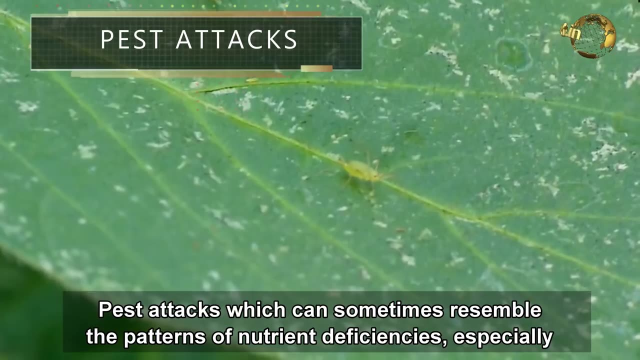 Most plants need a pH of around 6.0 for proper absorption of nutrients with the roots. Having this little pH meter will certainly help you rectify this problem. You can find related videos on altering the soil pH. 3. Pest Attacks, which can sometimes resemble the patterns of nutrient deficiencies, especially. 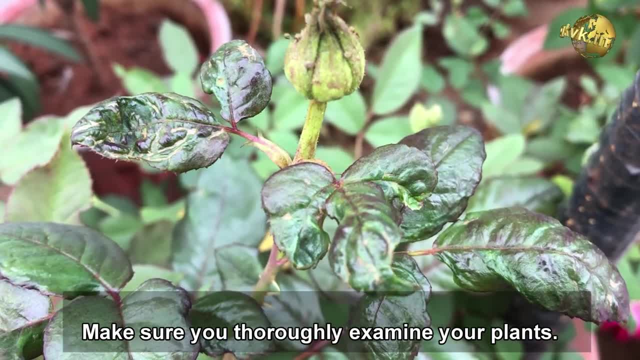 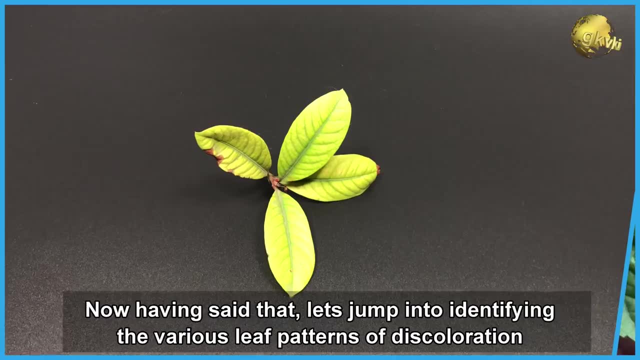 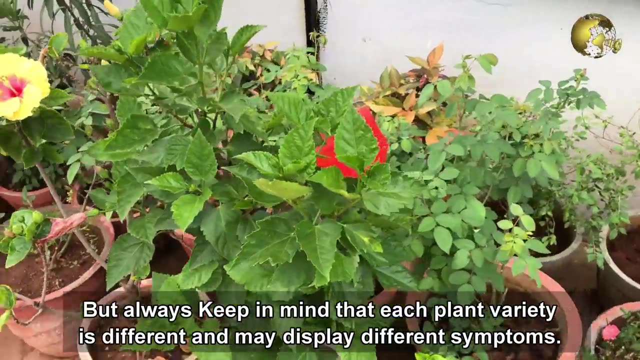 the sucking pests like aphids. Make sure you thoroughly examine your plants Now. having said that, lets jump into identifying the various leaf patterns of discoloration and distortion and diagnose this problem, But always keep in mind that each plant variety is different and may display different symptoms. 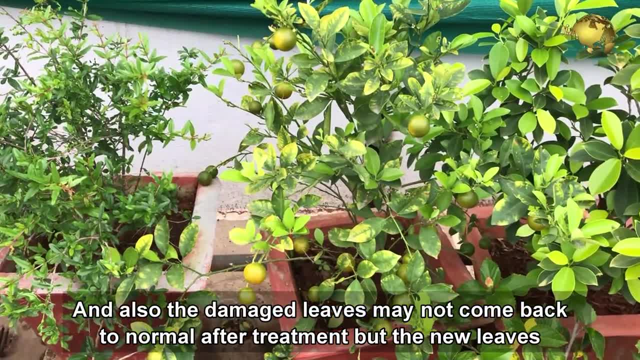 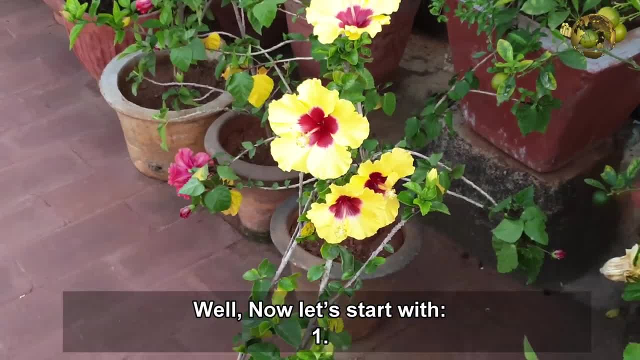 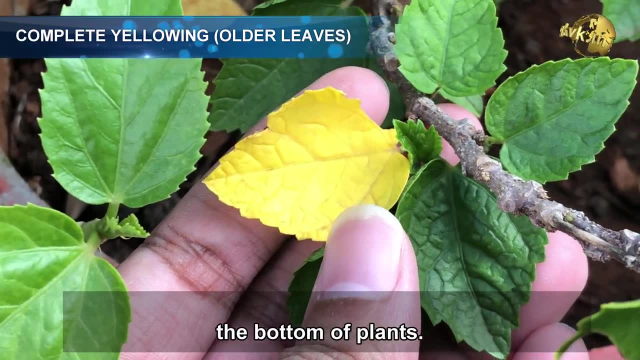 4. The damaged leaves may not come back to normal after treatment, but the new leaves will certainly come out healthy and lush after treatment. 5. Now lets start with Nitrogen Deficiency. You will notice complete yellowing of the older leaves, generally at the bottom of the 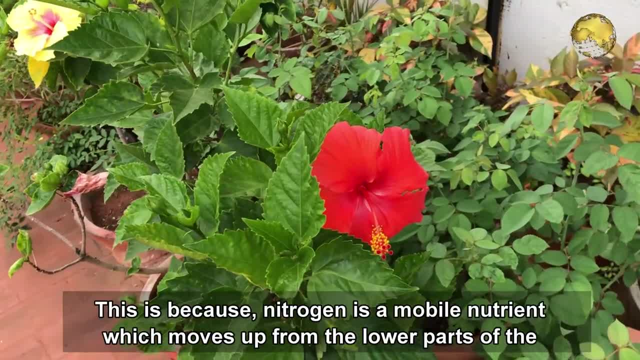 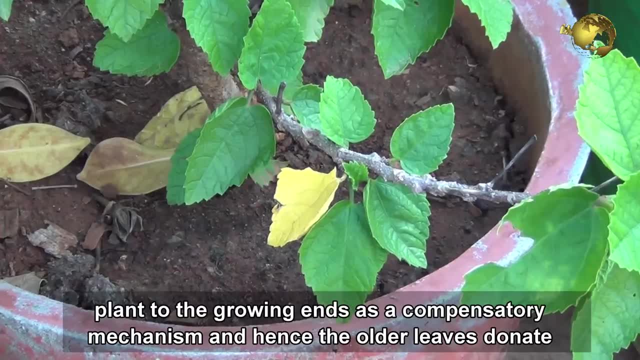 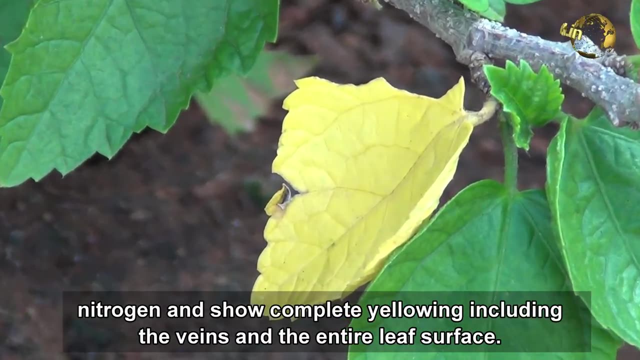 plants. The younger leaves are often healthy and green. This is because nitrogen is a mobile nutrient which moves up from the lower parts of the plant to the growing ends as a compensatory mechanism. 6. The older leaves donate nitrogen and show complete yellowing, including the veins and 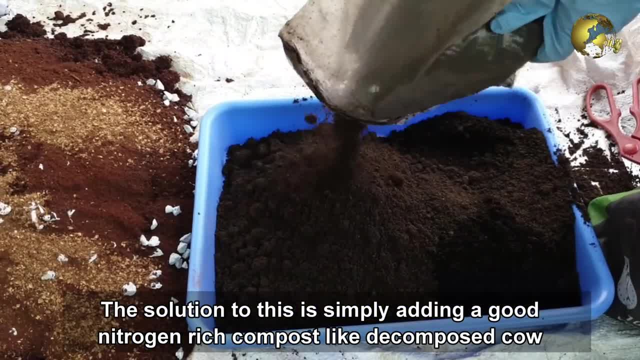 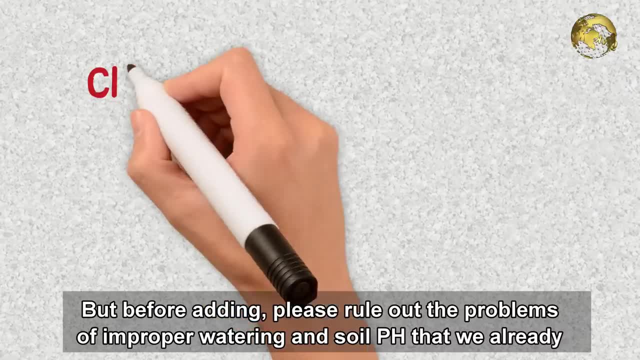 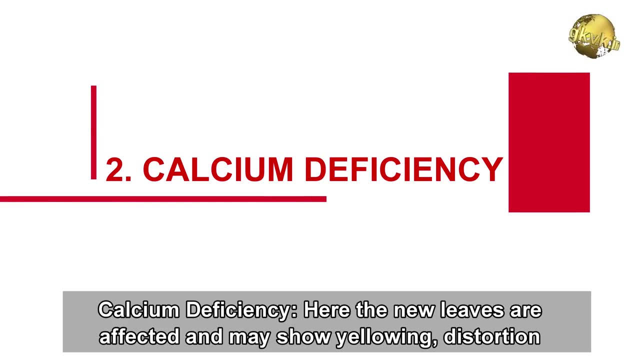 the entire surface. The solution to this is simply adding a good nitrogen rich compost like the decomposed cow dung or horse dung. But before adding this, please rule out the problems of improper watering and soil pH that we already discussed. 2. Calcium Deficiency: Here the new leaves are affected and may show. 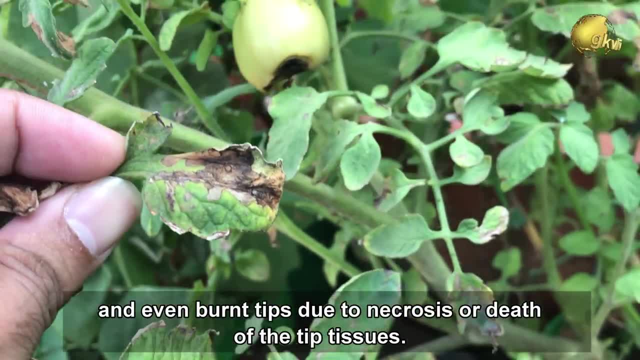 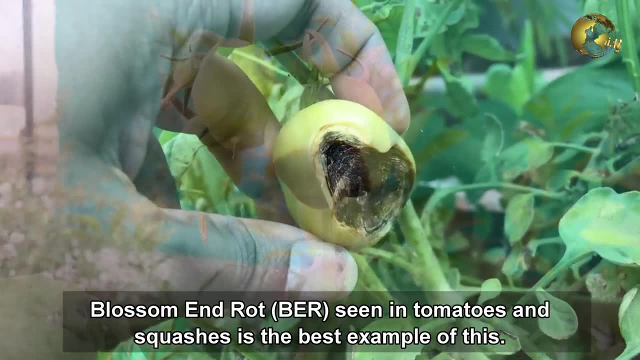 yellowing, distortion and even burnt tips. This is due to necrosis or the death of the tip tissues Blossom and rot. disease seen in tomatoes and squashes is the best example of this. We have discussed this problem and treatment in detail in my previous episode. 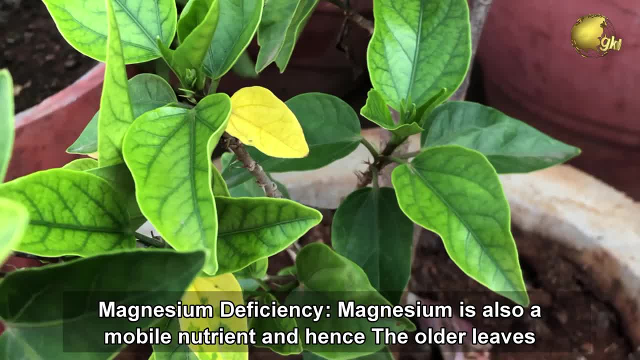 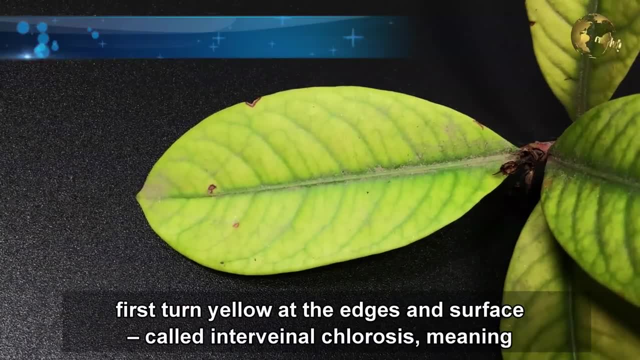 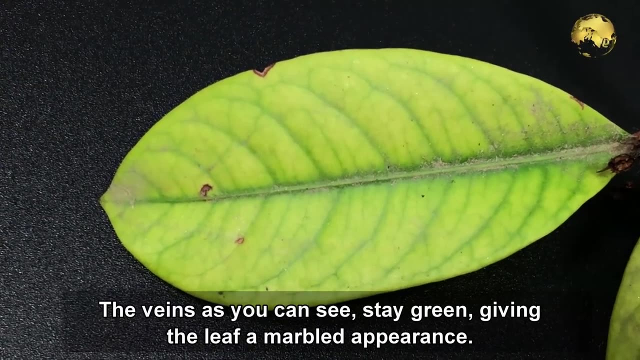 3. Magnesium Deficiency. Magnesium is also a mobile nutrient and hence the older leaves first turn yellow at the edges and the surface. that is called Intervenal Chlorosis, meaning yellowing between the leaf veins. The veins, as you can see, stay green, giving the leaf a marbled appearance. 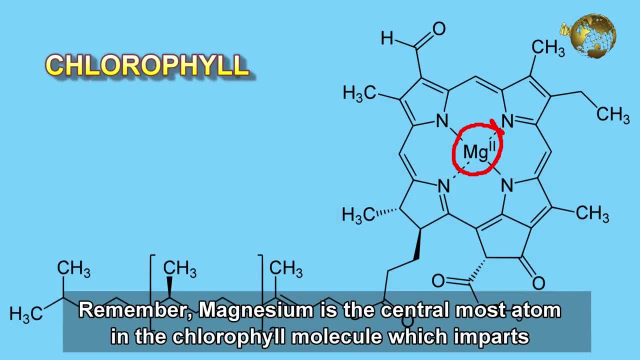 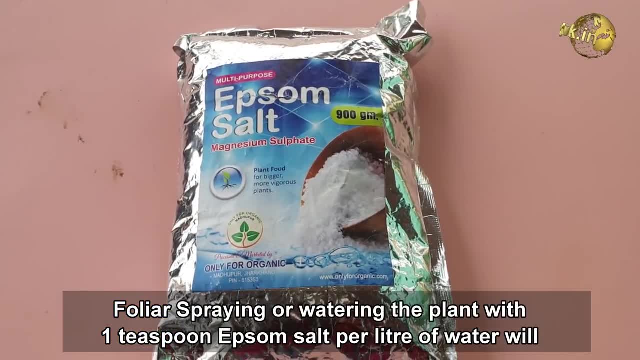 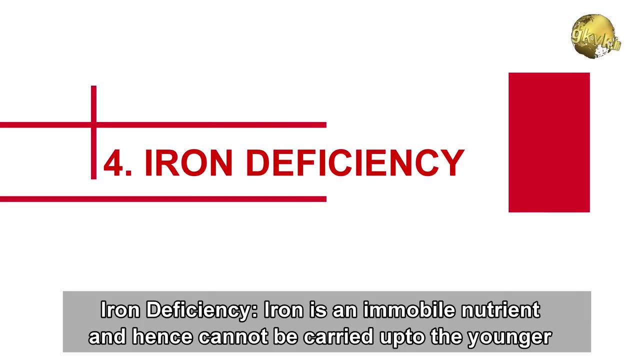 Remember, Magnesium is the central most atom in the chlorophyll molecule, which imparts green colour to the leaf Foliar. spraying or watering the plant with 1 tsp Epsom salt per litre of water will give great results. 4. Ion Deficiency: Ion is an immobile nutrient and hence cannot. 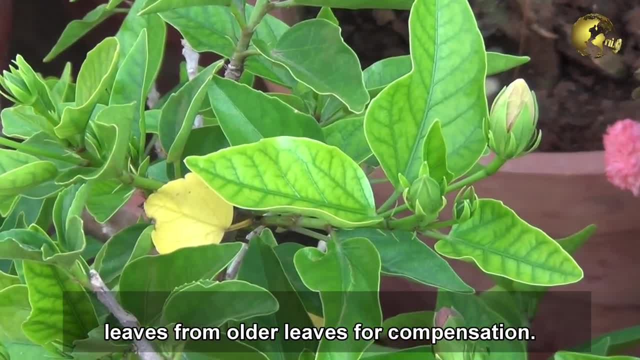 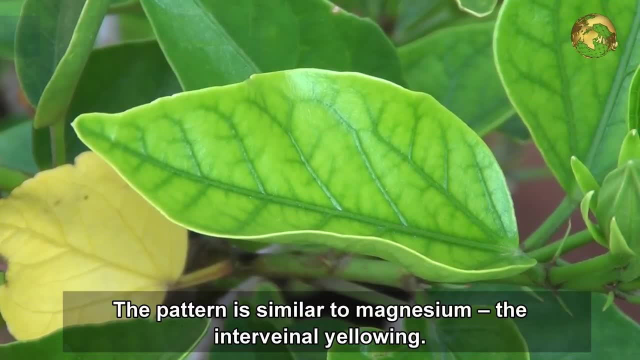 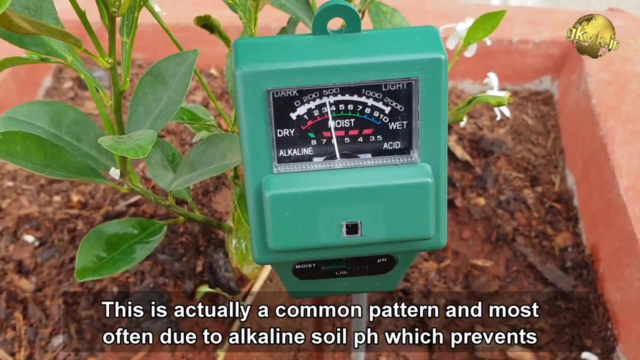 be carried up to the younger leaves from the older leaves for compensation. So the leaf yellowing is first evident at the tips or the younger leaves. The pattern is similar to Magnesium, that is the Intervenal yellowing. This is actually a common pattern and most often due to Alkaline soil pH, which prevents 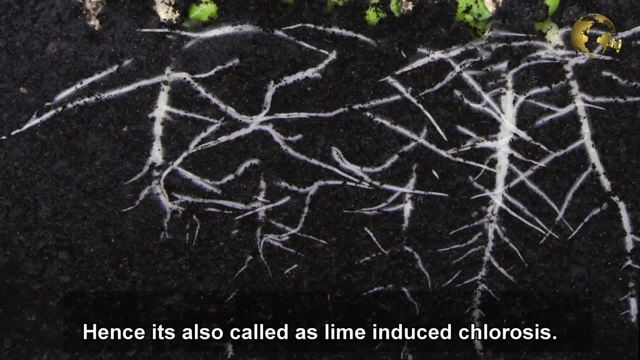 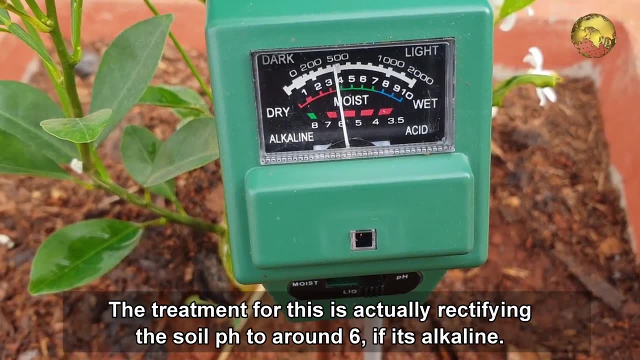 proper absorption of iron by the roots. Hence it is also called as Lime Induced Chlorosis. The treatment for this is actually rectifying the soil pH to around 6 if its alkaline. 5. Foliar Spray: Another method to bypass this problem is Foliar. 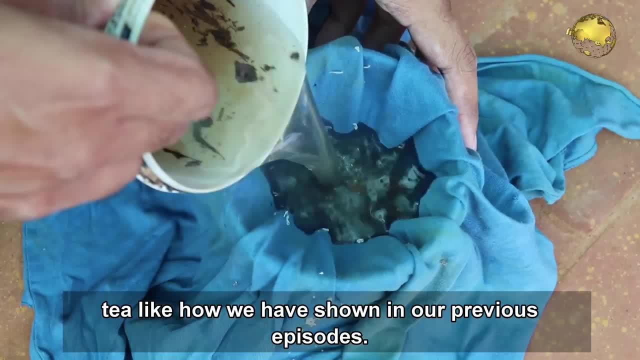 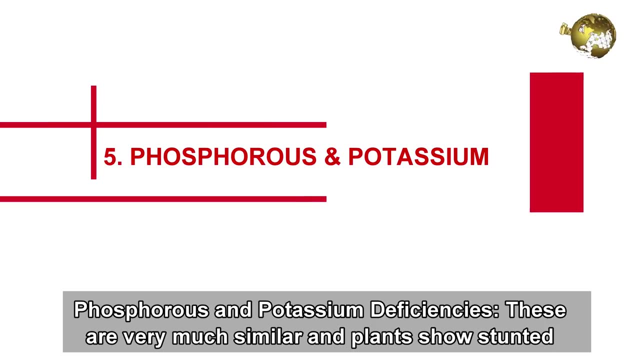 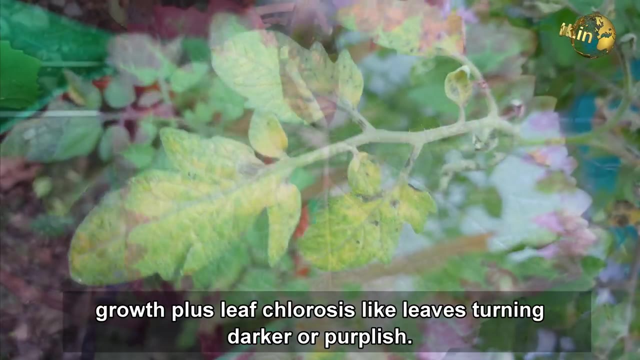 Spray of a micronutrient solution or even compost tea, like how we have done in our previous episodes. Related videos can be found in description links below. 5. Phosphorus and Potassium Deficiencies: These are very much similar to each other and the plants show stunted growth plus leaf chlorosis like leaves turning darker or purplish.